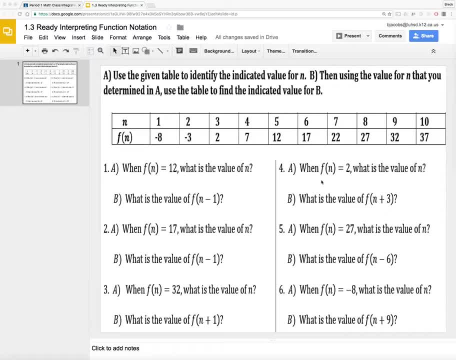 and paste it, place it in a slide so that we can type over this and annotate. So our job is to look at this table of values, right, And it says to find the value of n so that you could find the value of f of n. And so what's that mean? What's all this business? 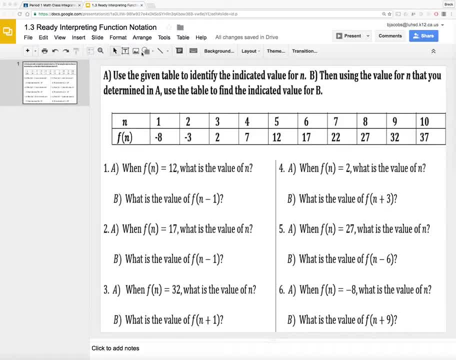 Well, we talked about this recently, about what a function is, and it's related to something we already know, And let me just create a box here so that we can see the information that I'm discussing, Since I don't have a highlighter. it'll be a box. 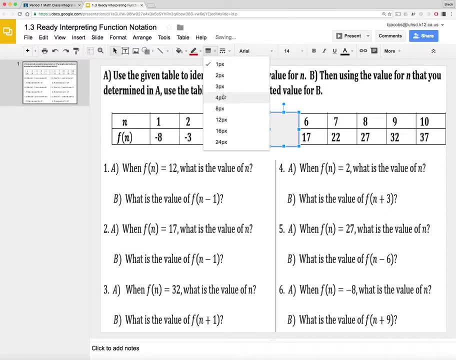 And that box will have a color and lines And I'll dash those lines And then I'll make the box transparent, Maybe a little larger than that. Let's go eight. Okay, So here's my box. See that right there. So let's look at five and two. What we know is those used. 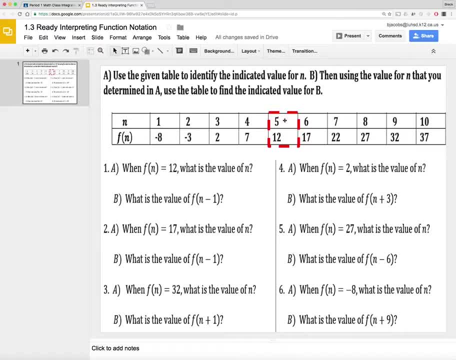 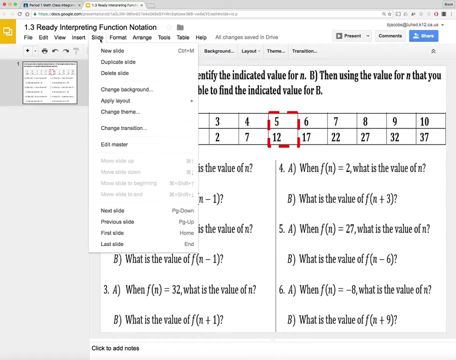 to be called the x and y values of your table, But we're no longer using x and y as describing these values. We're now using n and f of n, And so, in a sense, if I were to adjust these meanings, this would be your x value, the n and y would be your f of n. So, for the sake of clarity, 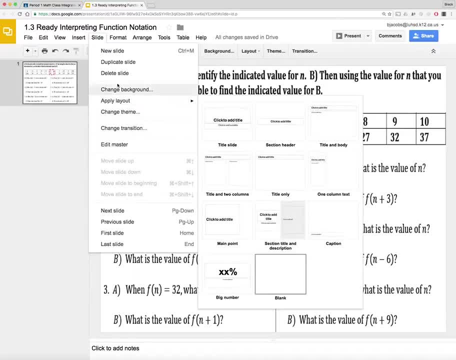 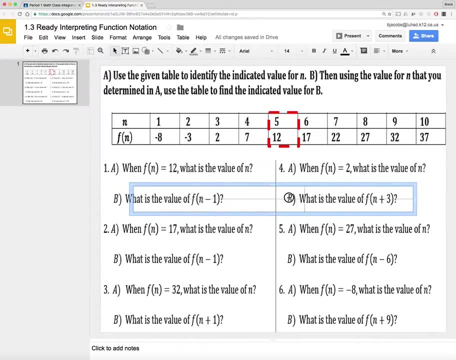 I want to make sure that you all know this. Let's go insert a table, Let's go just a single column, Two rows, And so this would be a lot like saying: let's enlarge this to maybe 24. again, This would be your x value And this would be your y value. 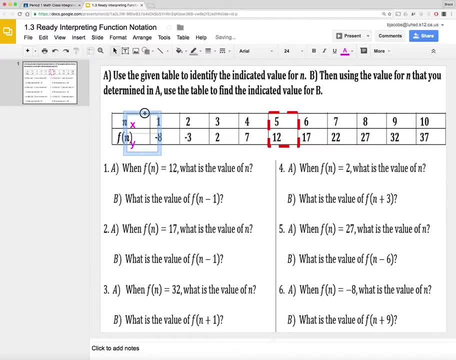 Okay, Okay. So let's look at this. So, when you have f of n equals 12.. So I just discussed, when you see something like f of n equals 12. What you are saying is that you're going to have y equals 12. And I'll scribble that on there Just for past reference. This is saying that 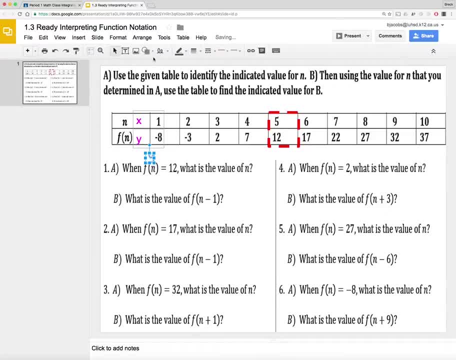 y equals. that's weird. That's my equal sign: Equals 12.. That's weird. That's my equal sign: Equals 12.. Okay, Okay, Okay, Okay, Okay, All right, All right. Well, that was not good. 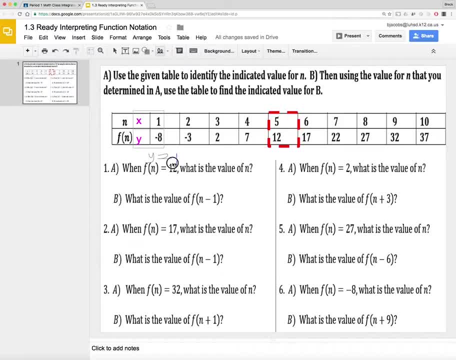 I hoped you could see it, But it seems we have it. Okay, And now. y equals 12.. You could see that we have y equals 12.. Well, we'll let me write 12, for some reason using the scribble. 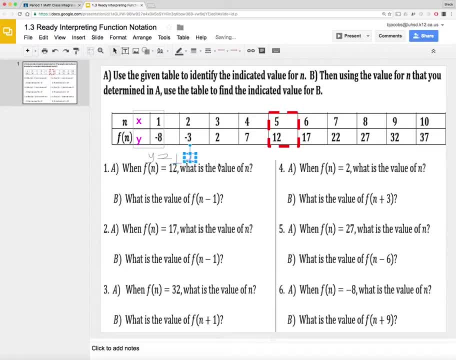 But y equals 12.. I'm not going to give up on this. There we go: y equals 12.. So what's the value of x? Well, where does y equal 12? at Here, Five 12.. When y equals 12.. 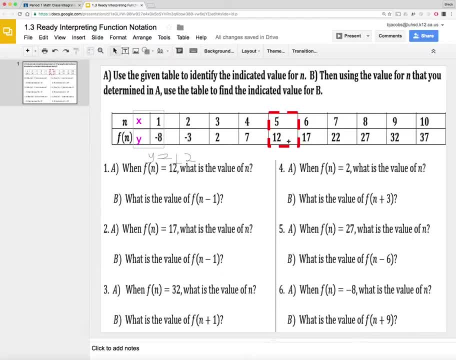 So what's the value of x? Well, where does y equal 12? at Here, Five, 12.. So when y equals 12.. y equals 12, the value of x is 5.. You see it, Instead of saying the value of x, we're saying what is the value of n? 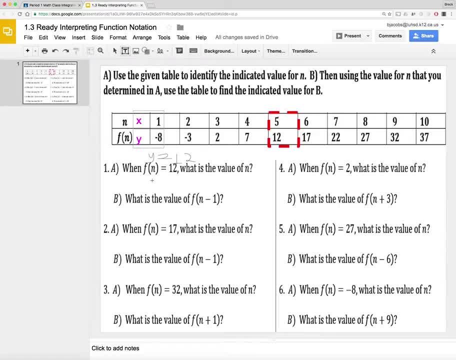 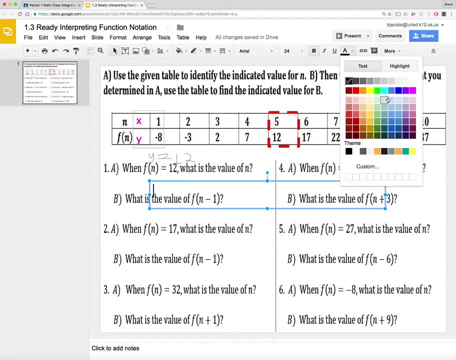 So the value of n is 5.. So let's type that in our text box. There's my value. Now for letter b says: what is the value of f of n minus 1? What's that mean? You say what is the value of f of n minus 1?? 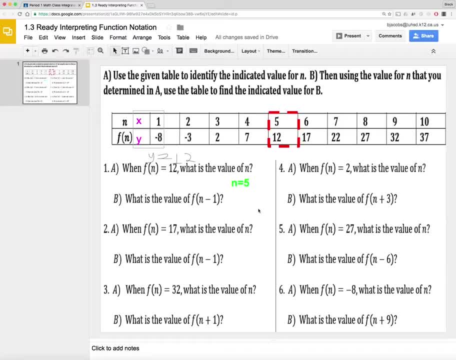 Well, when you subtract 1 from anything, it becomes smaller by 1.. And so what you're essentially saying here is that, hey, n is 5.. Right, Well, what's the value when n is 4?? Let me show you what that looks like. 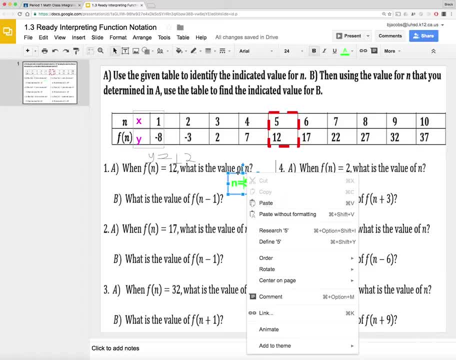 Watch this. Let's copy this here. So what you have here is this. Let's plug it in: See that: So 5 minus 1 is 4.. And what you're saying? there is what You're saying this. You're saying that, OK, 5 is here. 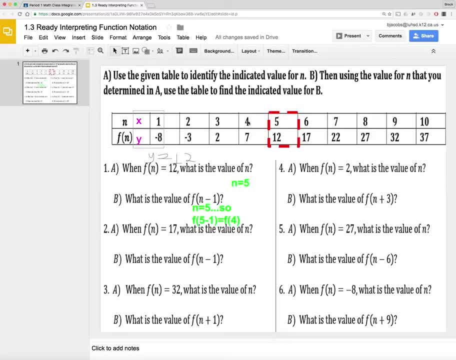 If you go back one spot right to here, see that right there That's 4.. And what's the y value? 7. 7. So we move back Back one unit, right Back one spot, to find the value of n equals 4.. 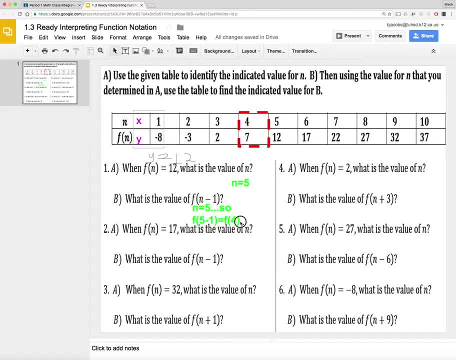 And now what's y, 7.? So we end up with 7.. So there you have it. So the key there is to take a good look at this and realize that's your answer. f of 4 equals 7. And our previous answer was here. 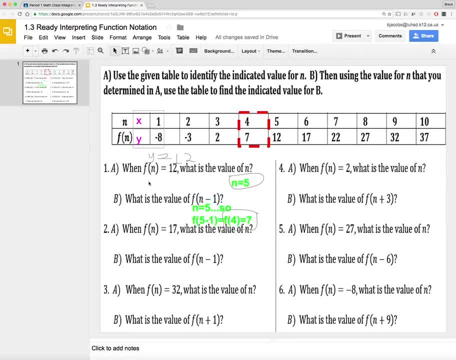 You see how that works. So you're going to be using the table of values to identify the information. f of n equals 12.. Where's 12? What's n? Oh, that's 5.. So n equals 5.. 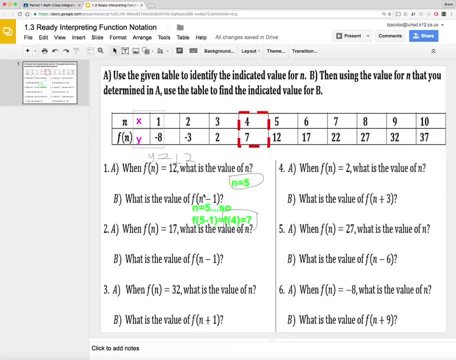 What is the value of f of n minus 1?? Oh, we know what 5, what n is: It's 5.. n is 5.. So 5 minus 1 is 4.. So f of 4,. go back to your table. 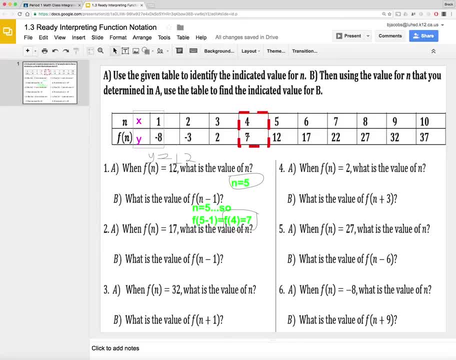 There's 4.. What's the output value? The y value, which we can now call f of n right, is 7.. And so you write that f of 4 equals 7, and there you have it. So I hope that helps. 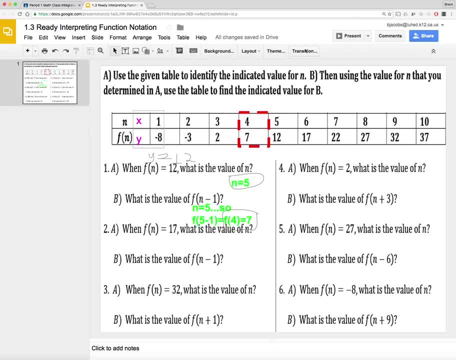 Try all these questions. Like I always say, study hard and learn a lot. We will see you soon.